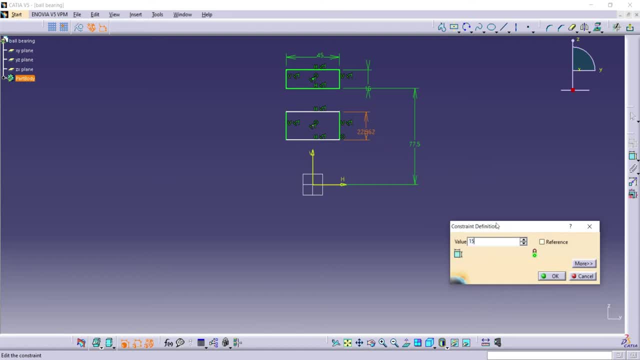 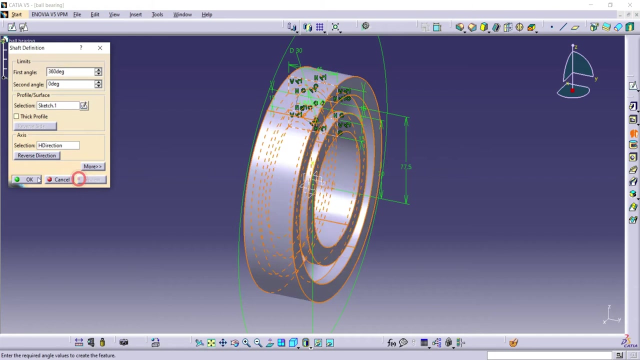 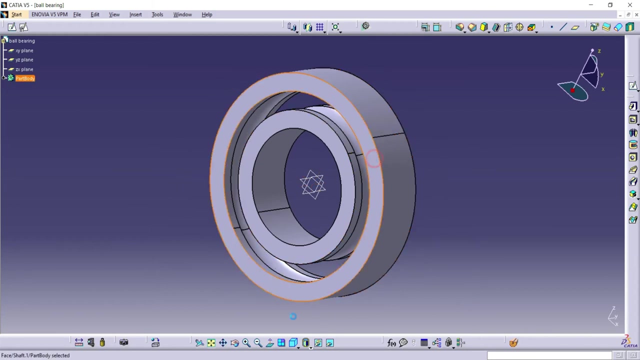 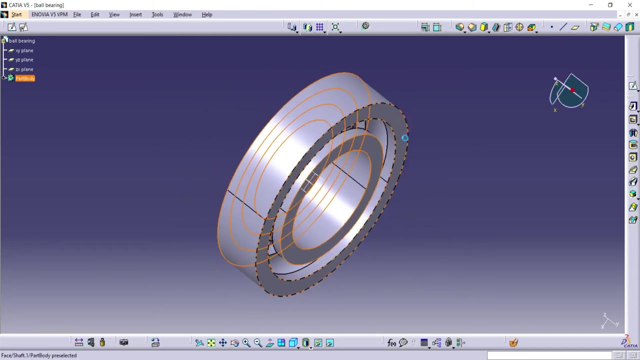 But to look easier and have the ability ofществ to write theOO in Hit desk, Maybe in some cases can design the print in the printer. Please "' athletics toright now' Thank you. Use sharp tool to make the sketch solid. Use edge fillet to make smoother edges. 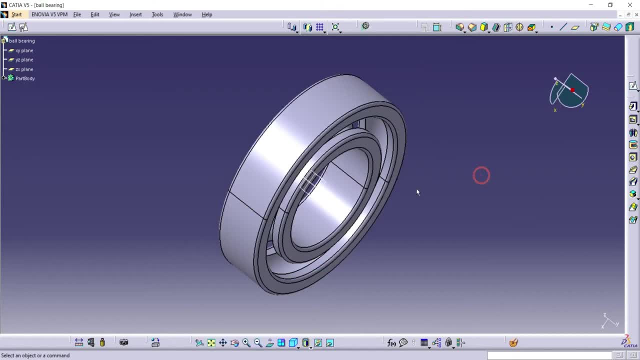 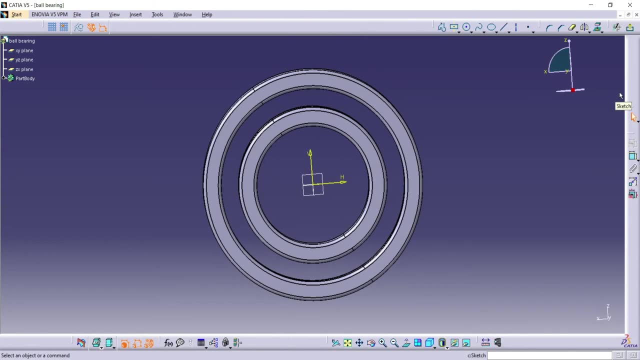 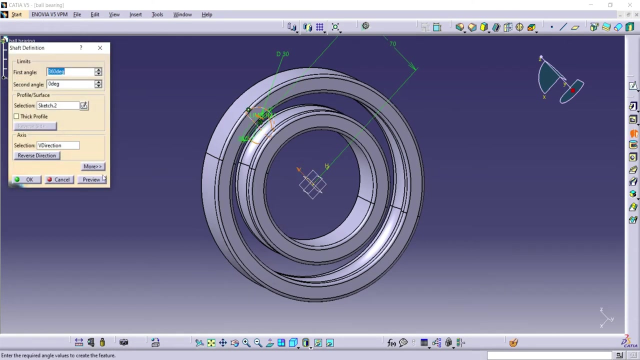 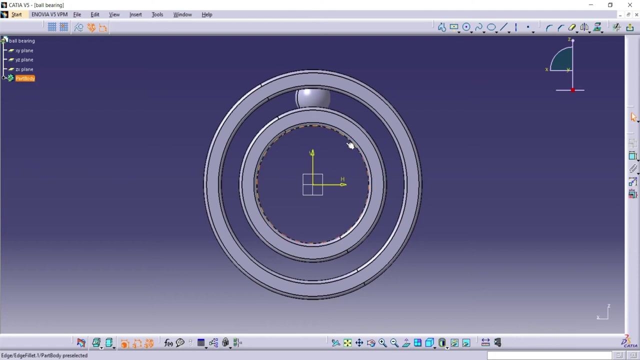 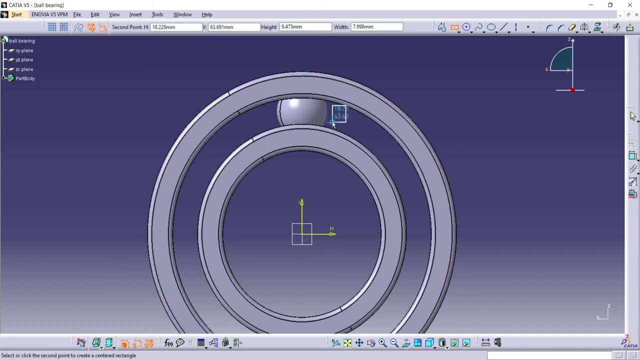 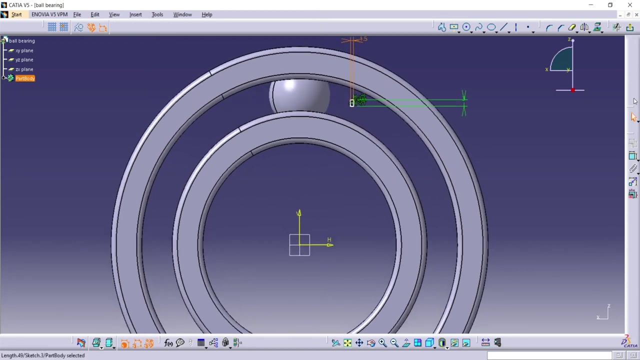 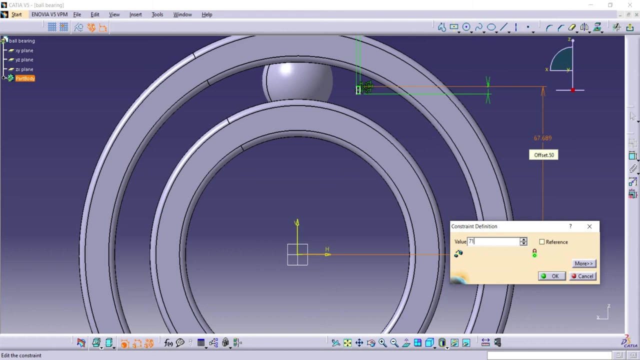